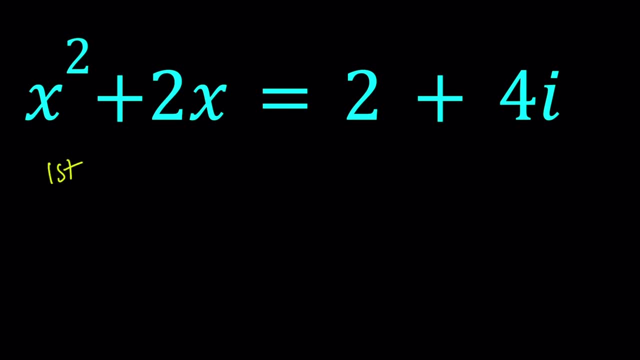 start with the first one. So for my first method, since this is quadratic, I'm going to collect everything on the same side and then use the quadratic formula. Let's see how that works: x squared plus 2x. and then I'm going to subtract 2 plus 4i. Let's go. 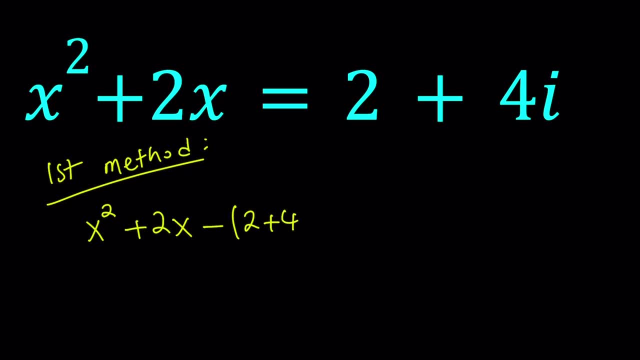 ahead and subtract the whole thing as an entity like this and set it equal to 0.. Notice that in this equation, negative, the negative of 2 plus 4i- is our constant term, because i is a constant right, Even though it's imaginary, complex, whatever, it's a constant It's not. 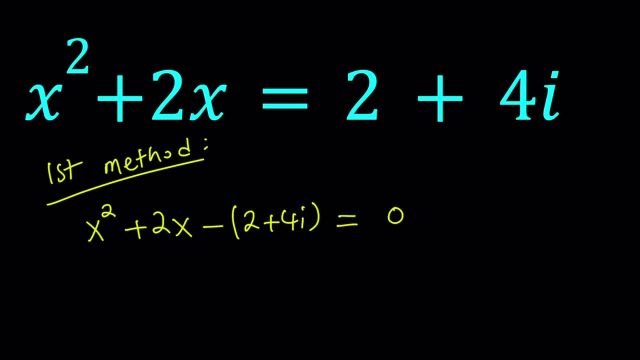 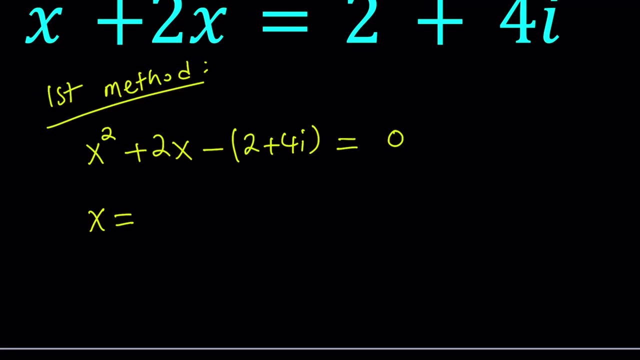 a variable. So we can use the quadratic formula. since this is quadratic, x equals and that's going to give us the following: Remember the quadratic formula: If you have ax squared plus bx plus c equals 0, then x is given by negative b plus minus. 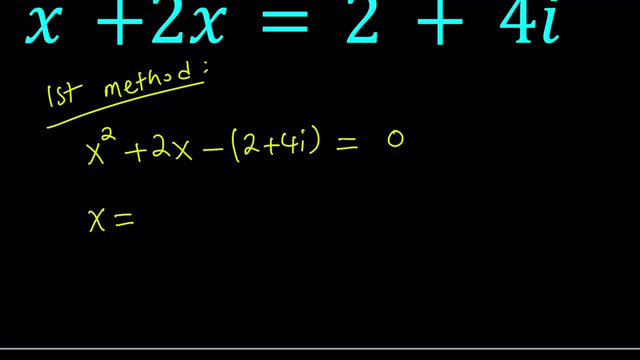 The square root of b squared minus 4ac all over 2a. So negative b plus minus the square root of b squared, which is 4, minus 4 times a1, which is not going to matter here, We don't need to write it. Times c, c has a negative sign, so the double negative is going to make. 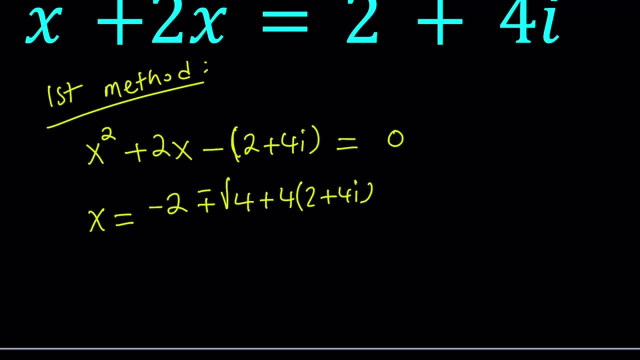 it a positive, And we can just multiply 2 plus 4i by 4.. And then divide the whole thing by 2a, Which is 2.. So let's go ahead and simplify this expression and see what we get from here. 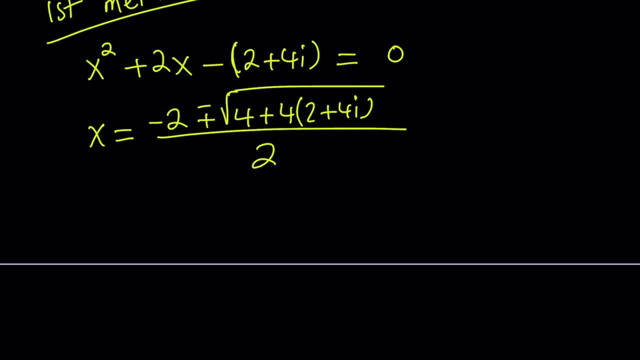 So how do you simplify inside the radical? Let's go ahead and do that We're going to multiply, distribute and simplify. 4 plus 4 times 2 is going to be 8.. And then 4 times 4i is going to be 16i, And then just we're going to divide it by 2.. Now, if you combine, 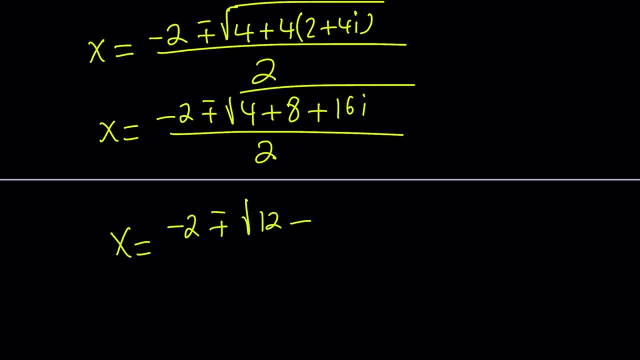 like terms inside the radical. you're going to get the following: You're going to get 12 plus 16i, And all of that is divided by 2. Awesome. Now here's the most important part: How do you square root 12 plus 16i? That's just going to be. 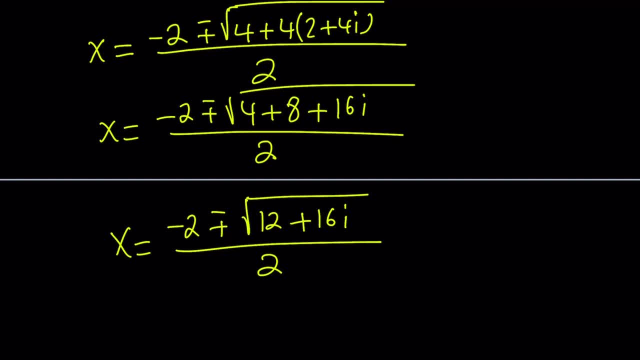 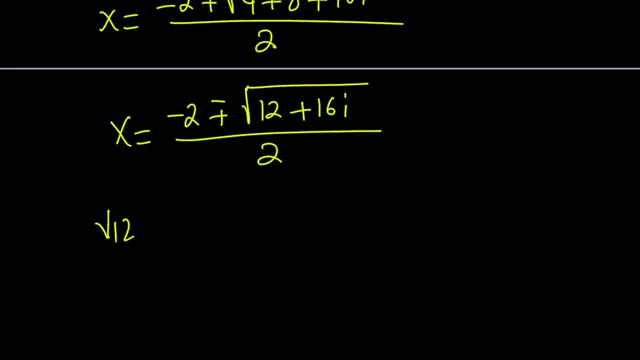 another problem in and of itself, But if you kind of think about it, there's a couple different ways to go about it. You can set it equal to. so, if you're trying to square root this number, I'm going to draw out a 2, which is, I mean, not a 2,, a 4, which will come out as a 2.. 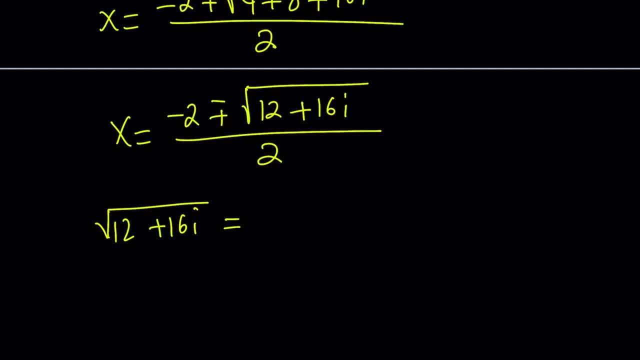 So it's going to be like this: Let me take out a 4 here, and then I'll show my work, And then, if you take out the 4, it's going to be a 2.. So we're just going to square root. 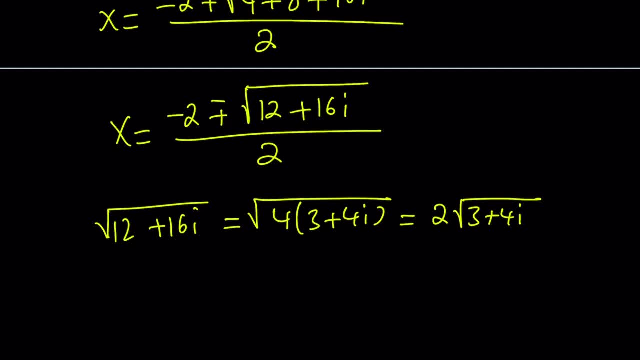 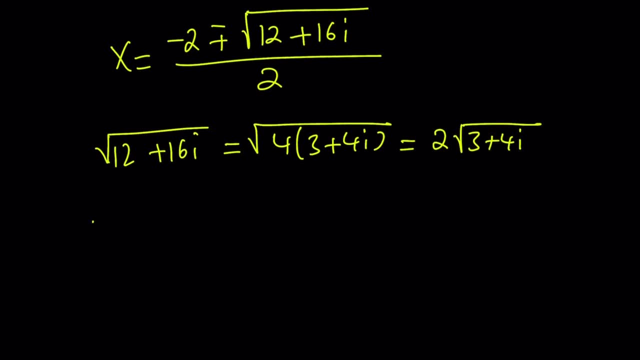 3 plus 4i. How do you square root 3 plus 4i, Right? Okay, Here's what you can do to simplify it. You can set this equal to. you can set this equal to a plus bi And then square both sides. 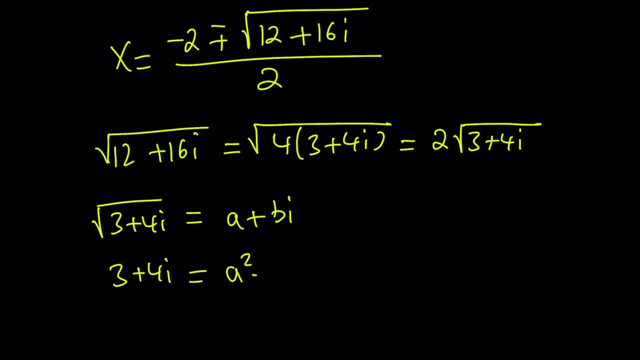 And then that's going to give you a squared plus b squared. i squared, That's just going to be a negative b squared plus 2abi. Here we have to set the coefficients, or real parts to real parts and imaginary parts to the imaginary parts. So it's going to be like this: a squared. 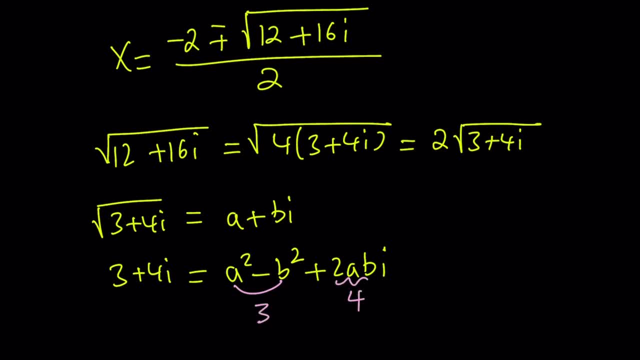 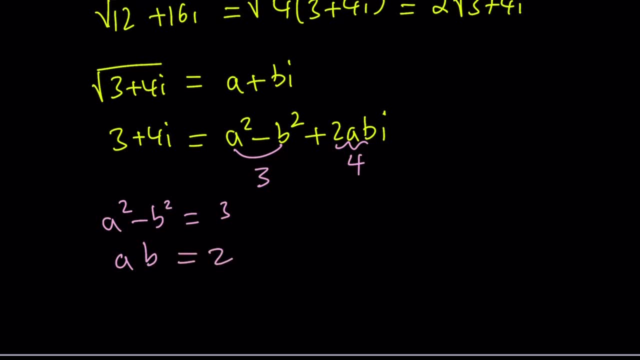 minus b squared is going to be a: 3. And 2ab is going to be a 4, which means ab is 2.. So a squared minus b squared is 3 and ab is 2.. So kind of think about two numbers whose. 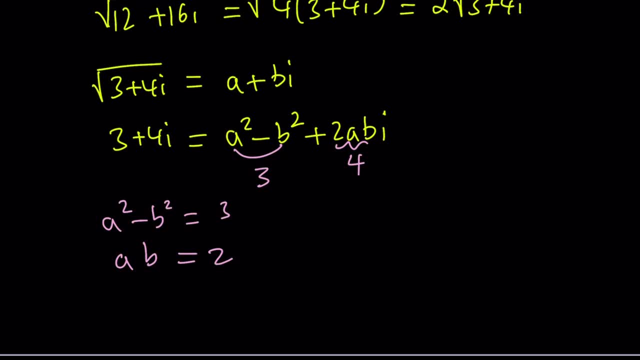 product is 2 and whose difference of squares is 3.. And I'm hoping that you can easily find that those numbers are 2 and 1.. And of course, negative 2 and negative 1 is also going to work. But we already know that if we can find one of the square roots, then the other one. 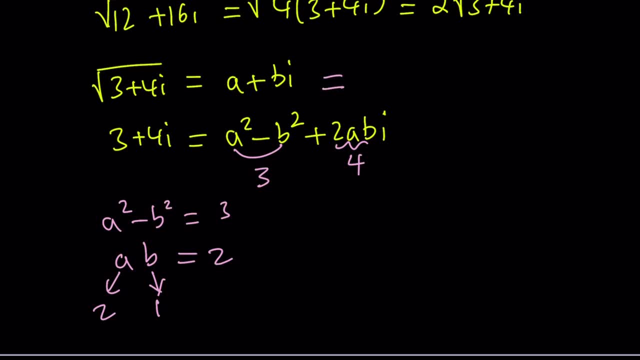 is going to be fairly easy. So a plus bi from here becomes 2 plus i. You could also arrive at the same answer by manipulating 3 plus 4i. You could kind of write it like 4 minus 1 plus 4i and then write: 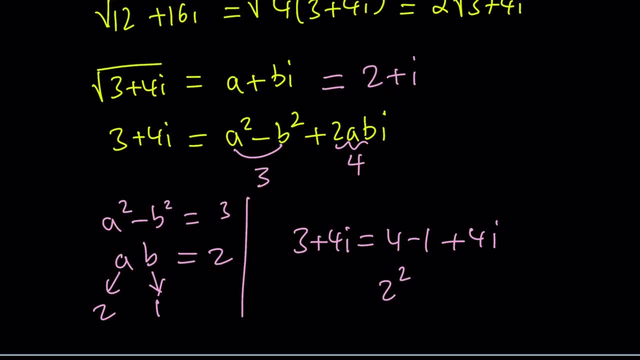 the 4 as 2 squared, and then write the negative 1 as i squared, and then write this as 2 times 2 times i, And then you can kind of make it a perfect square, right? Okay, there's a couple. 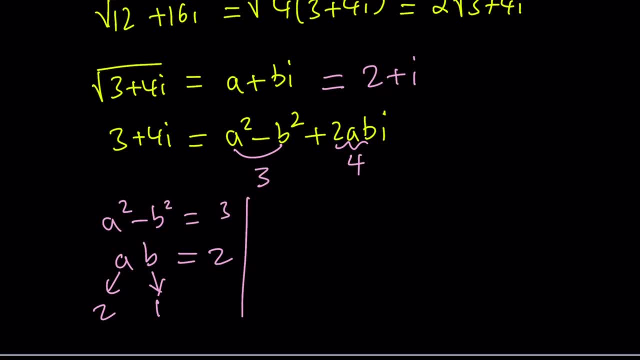 different ways to go about it, Since this is a nice one, you can easily find it. But what if I told you: okay, can you find the square root of 7 plus 5i? It's not going to be that straightforward. Then you have to solve this equation. okay, Great, So there's obviously a 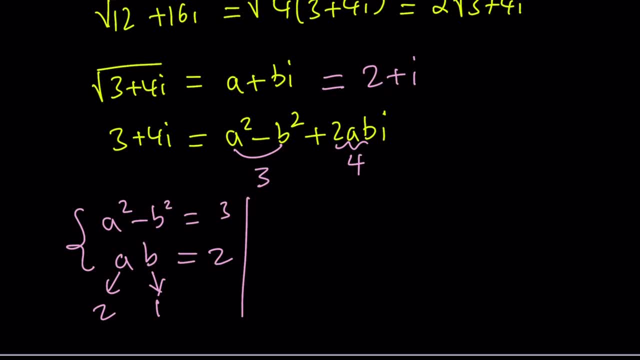 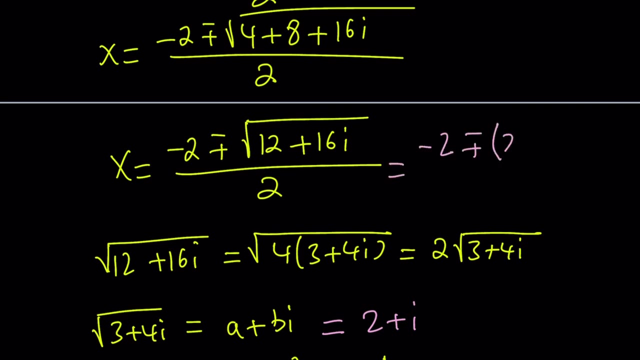 general method, as well as a formula which we can probably talk about now. Maybe I can share that in a post, because that's really cool, Anyways. so we got one of the square roots, which is 2 plus i, So we can go ahead and plug it in here: negative 2 plus minus 2 plus. 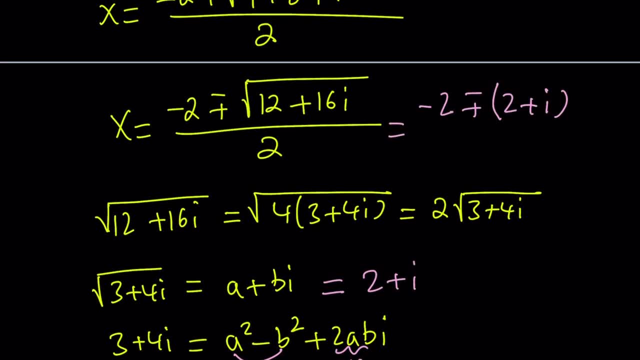 i, That was the square root right All over 2.. And obviously we can go ahead and combine this, but notice that I'm going to clean up the bottom so I can continue here. We can go ahead and square root it. I mean not square root it, Let's just combine them. but there's a plus- minus sign. 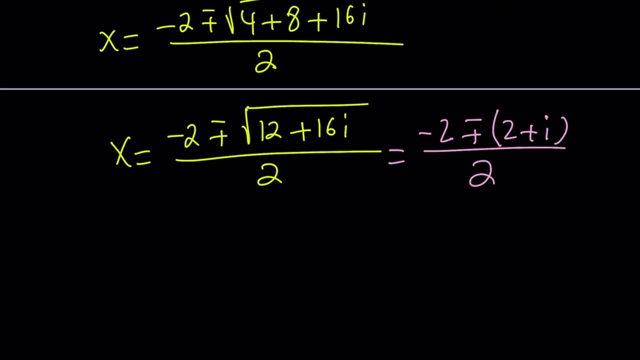 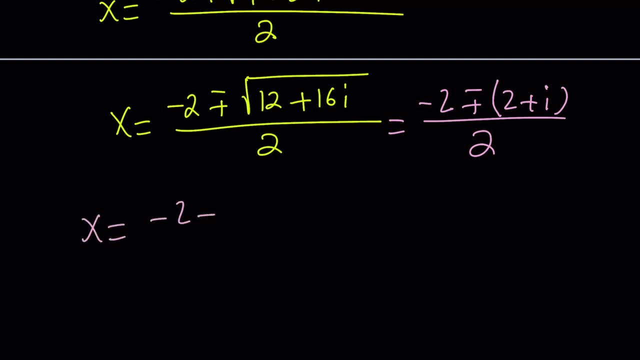 So we're going to consider two cases, because we have two solutions right? This equation is quadratic and it has two solutions, So one of them is going to be: x equals negative 2 plus 2 plus i divided by 2.. 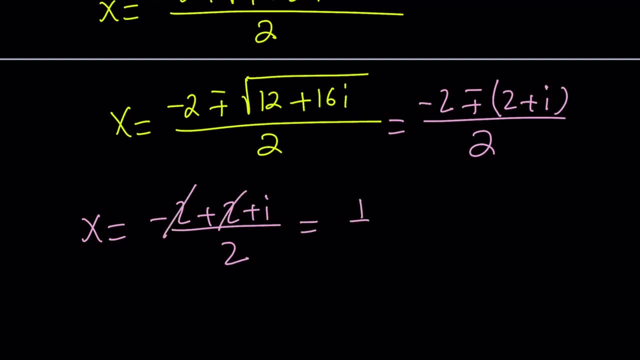 Negative. 2 and 2 is going to cancel out. We're going to get half of i, okay. Oops, I forgot one thing. I just realized there was a 2 in front of the radical, so I need to write that as well. So, 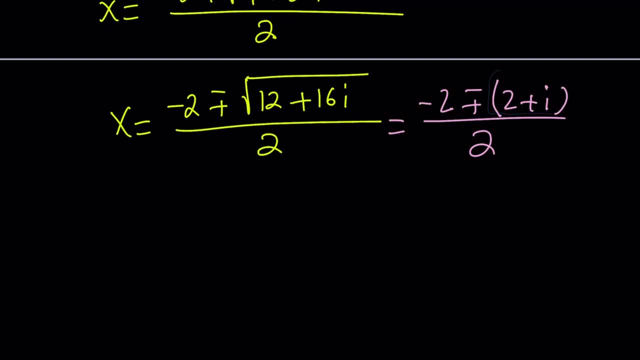 let's go ahead and see if I can do this real quick. I want to move this a little bit to the left, to the right, I mean, and then fit the- what is it called? The 2 in there. Here you go. So x is. 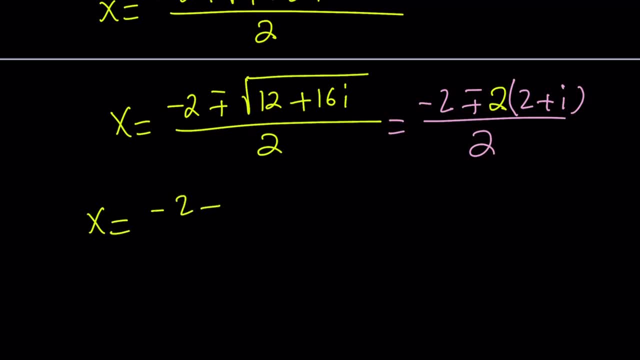 going to be negative: 2 plus minus. I should probably just keep the 2 inside, Anyways. so if you go with the positive solution, okay, let me write it. This didn't look good, So x can be written as okay, let's just go with. 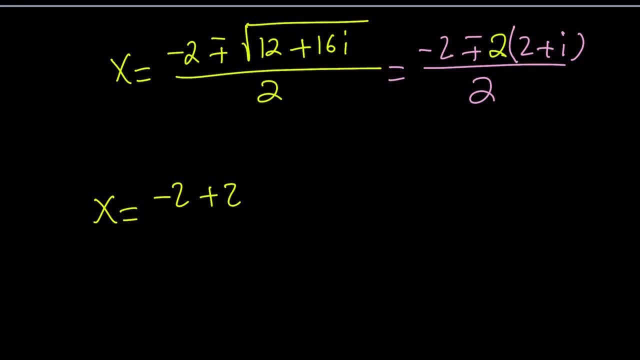 the positive first Negative: 2 plus 2 times 2 plus i divided by 2.. That's going to be negative 2 plus 4.. That's going to be a 2 plus 2i divided by 2, which is going to be 1 plus i And the other. 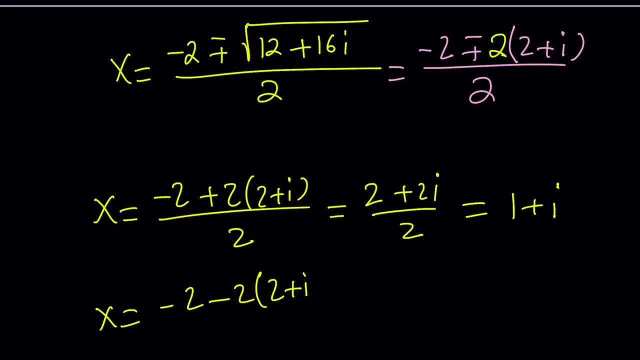 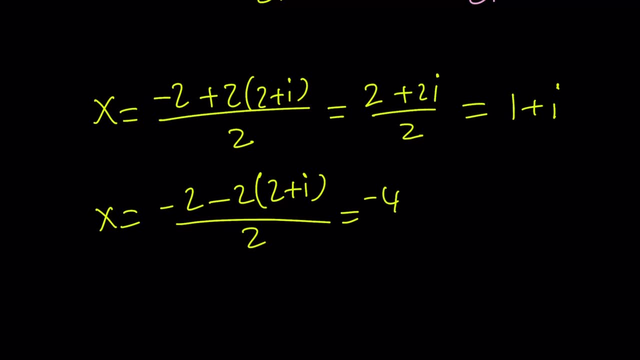 solution is going to be negative 2 minus 2.. 2 plus 2 times 2 plus. i. Make sure to keep the minus outside the parentheses so you can distribute it. It's going to give us a negative 2 minus 2, negative 4 minus 2i divided by 2, and that is.